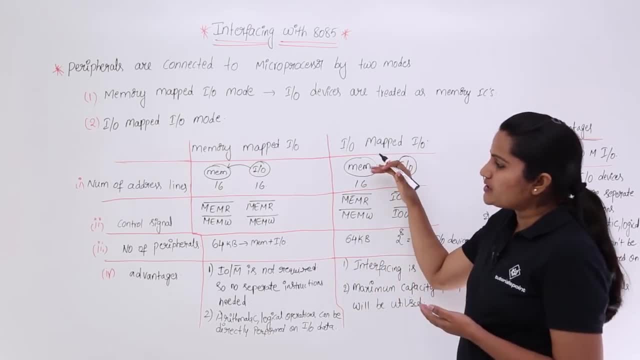 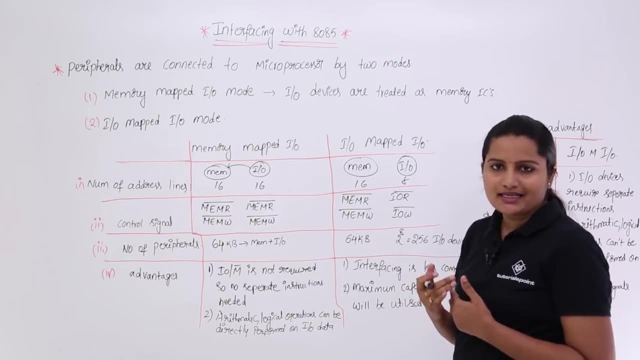 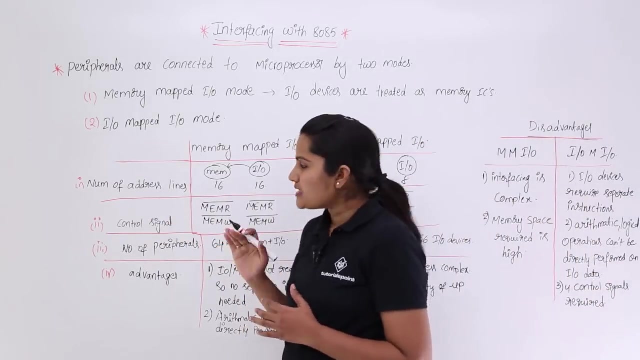 memory. So coming to I-O mapped I-O mode, for memory we are using only 16 address lines and for I-O we are using 8 address lines. So here for I-O we are using less address lines and for memory we are using all 16 address lines. Coming to control signals, as we are using I-O is also. 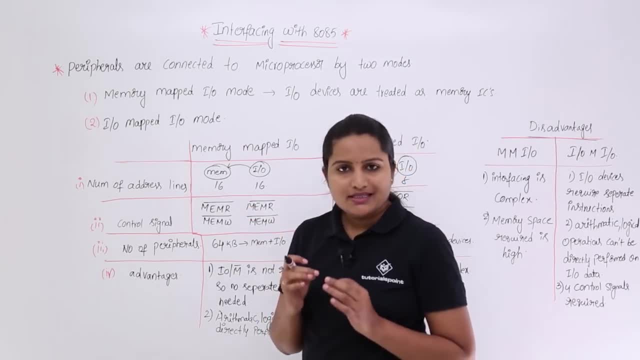 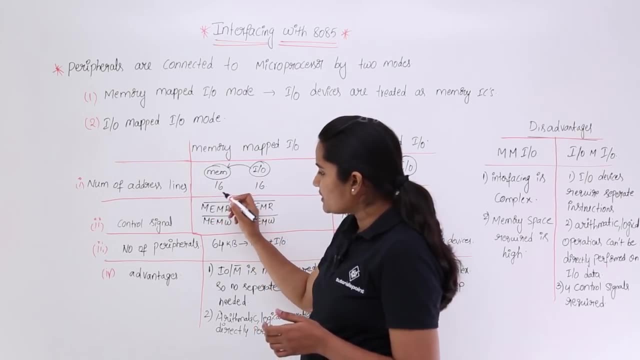 as memory chip. we are using same control signals which are using for memory. That means to control this memory. whatever You are using, same signal we are using for I-O because we are using I-O as memory only. So here, 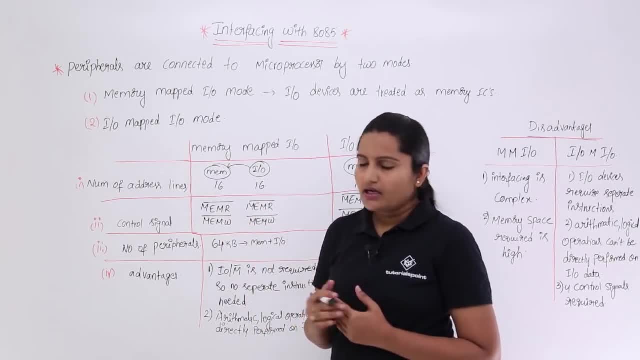 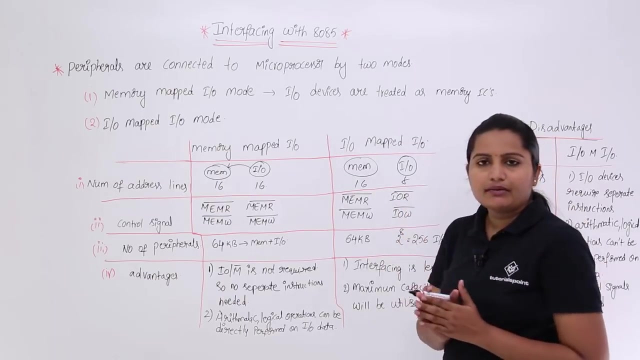 M-E-M-R refers to memory read and M-E-M-W stands for memory write. These read and write control signals are used for both memory and I-O operations. Now coming to this I-O mapped I-O here, as we are taking memory and I-O separately, here we are having four different control signals. 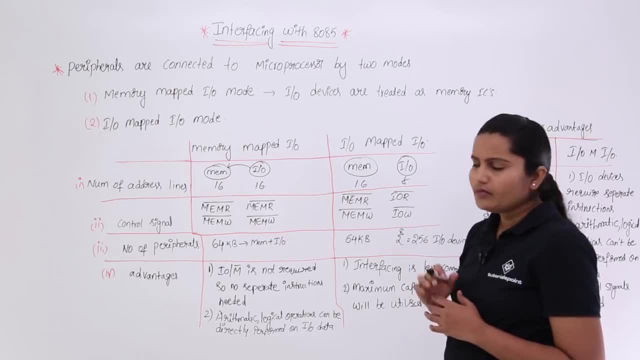 For read and write of that particular memory and I-O. You know that to read or write the memory you require M-E-M-R bar and M-E-M-W bar, But to read and write I-O you require I-O-R bar and 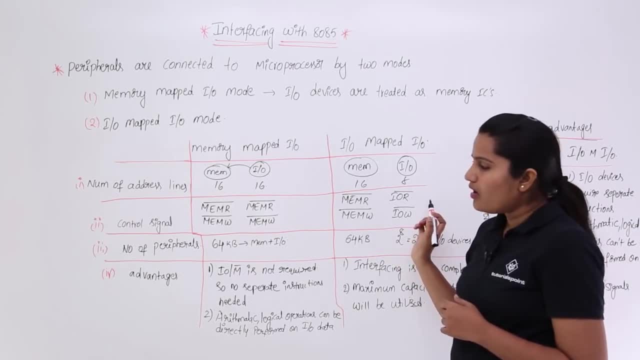 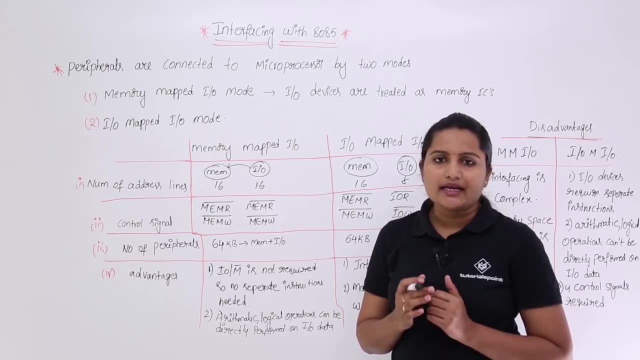 I-O-W bar. That means I-O read and I-O write. All these control signals are active low. If you observe these signals, you can identify a bar, So that means those are active low. Whenever they got zero at its input, they are going to control the memory, So that means those are. 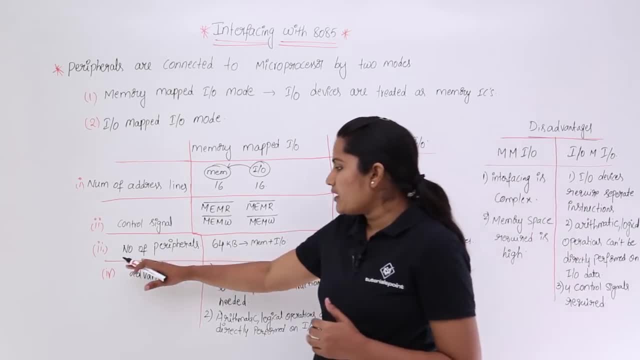 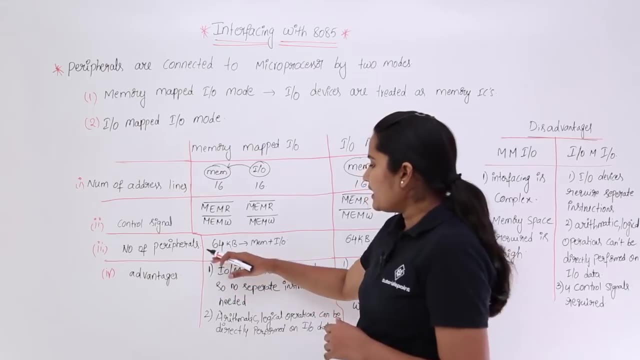 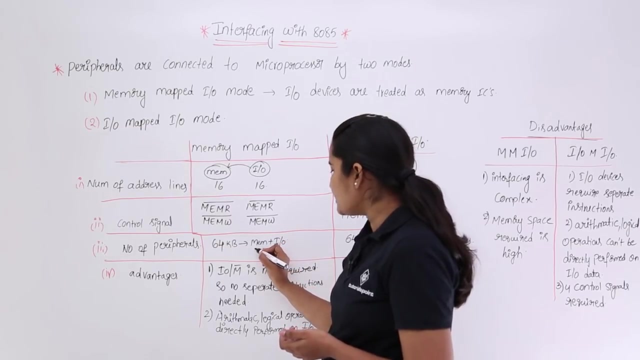 going to control a particular operation. So now, number of peripherals. Coming to the number of peripherals, So it can be dependent upon the size, So we can connect up to 64 KB, So both for memory and I-O. For example, if your memory interfacing is 64 KB, you need to consider I-O as 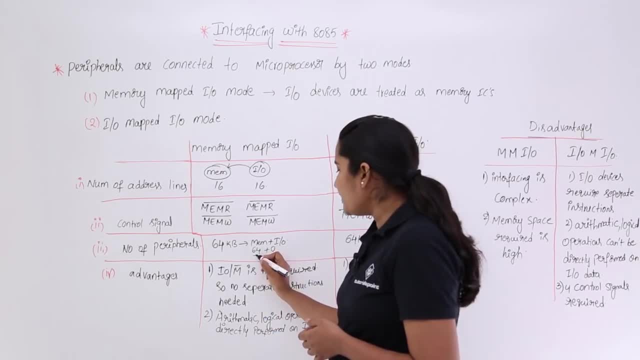 zero. For example, if you are taking 50 for memory, so you need to consider remaining 14 for 14 KB for I-O, So like that you can connect up to 64 KB. So that means you can connect up to. 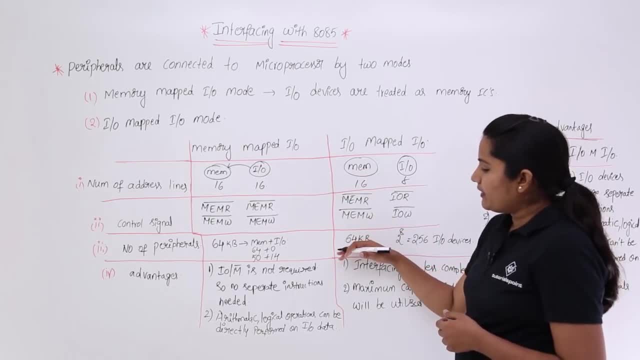 64 KB. So coming to here, So for memory we are having 64 KB. So for I-O we have access up to 2 power 8. That means 256 I-O devices we can connect. So 256 I-O devices we can connect. 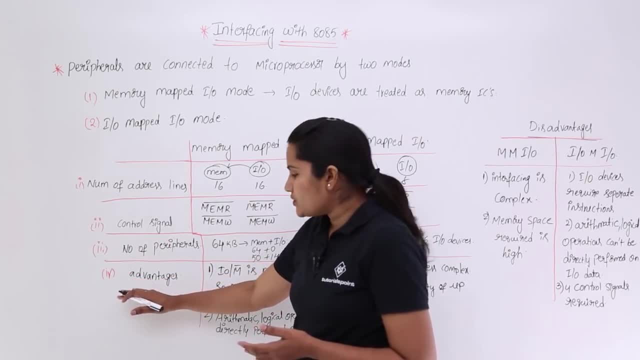 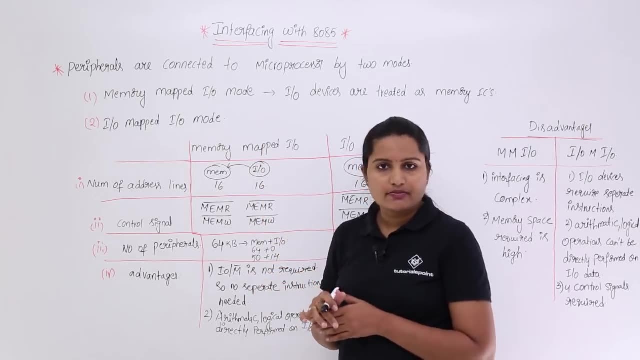 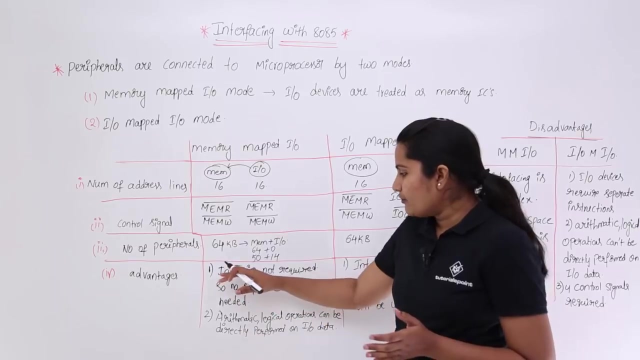 So now coming to number of advantages. So coming to advantages here. you know that you are not using your I-O. I-O is also used as memory in memory mapped I-O mode. As you are not using your I-O, so then I-O M signal is not required. Why? Because 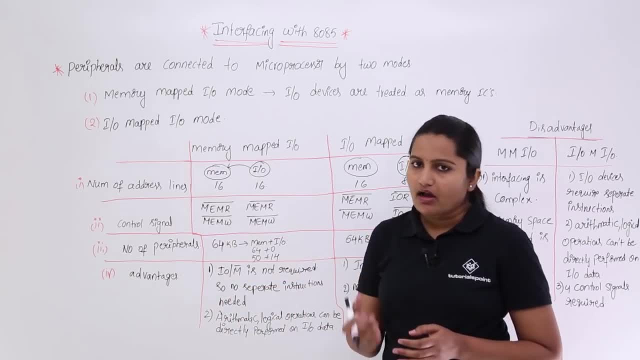 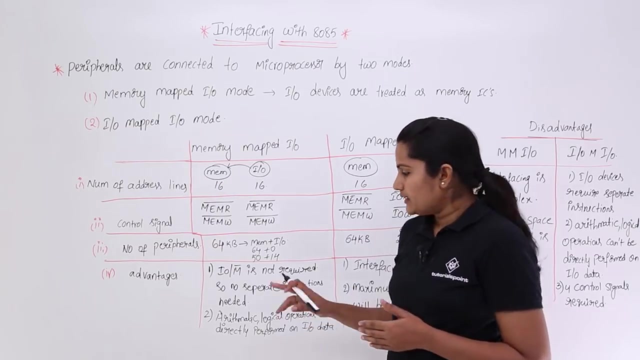 so generally this is a signal to identify the writer. read operation is related to either I-O or memory. Here I-O and memory, both are used as memory means no need to identify whether that equation is related to that I-O or memory. then definitely your I-O and M bar signal is: 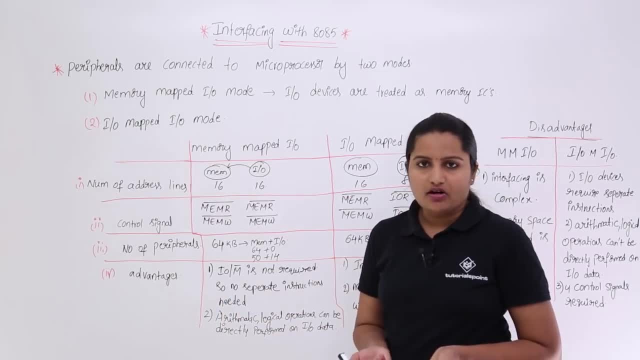 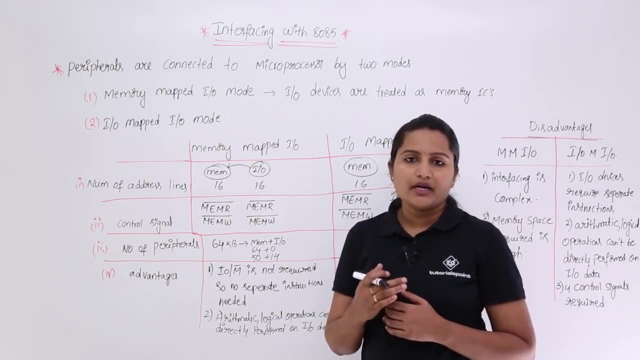 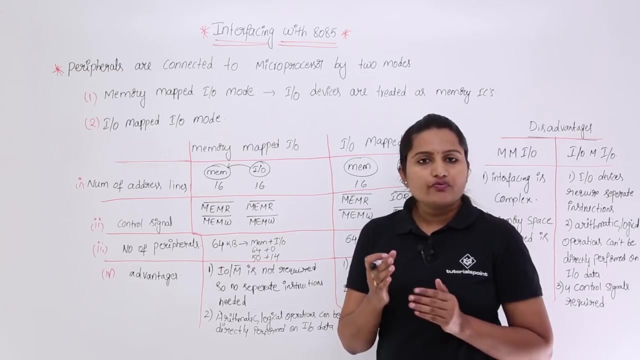 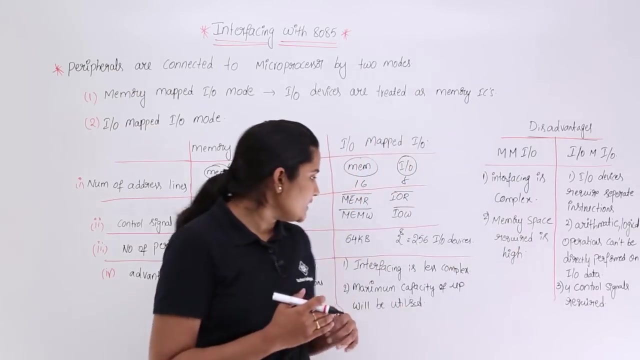 required. so separate instructions are not required. so that implies separate instructions are also not required. second advantage is arithmetic logical operations we can directly perform on io data. so as we are using io as memory directly, so we can perform arithmetic and logical operations on io data directly. so coming to the advantages of this, io mapped, io mode interfacing is 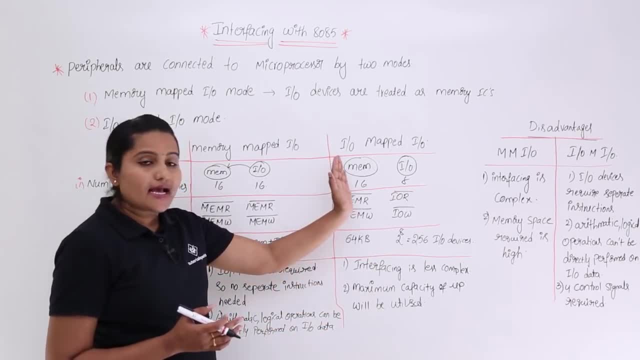 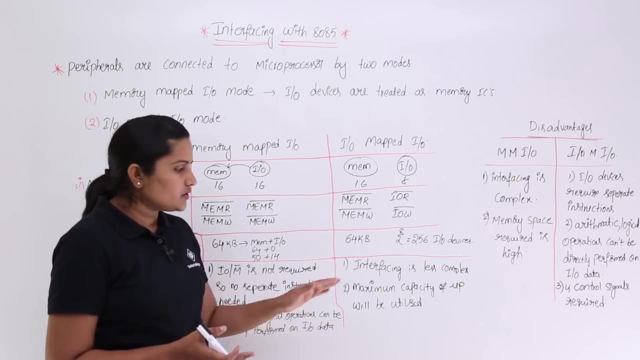 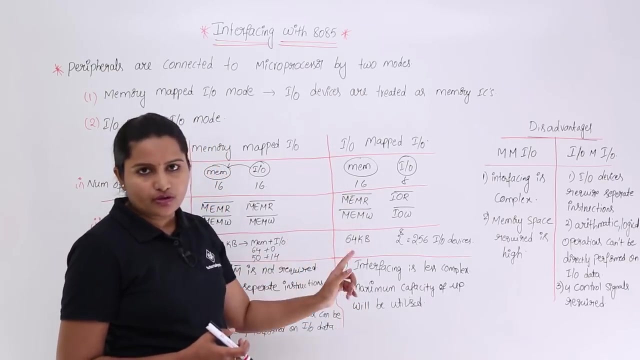 less complex. so that means. so here, as we are using separately, we are having some clarity. so interfacing is not that much complex. so this is less complex for interfacing and maximum capacity of microprocessor is utilized in this mode. so now coming to the disadvantages of both modes, 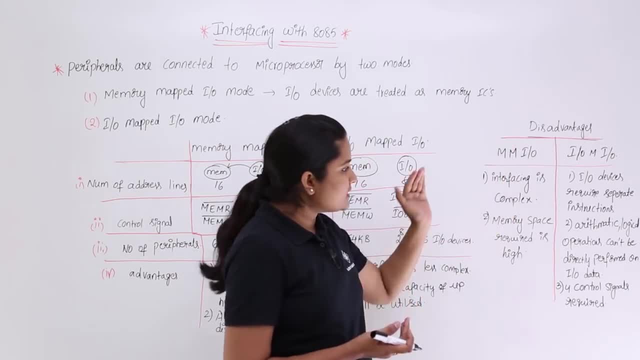 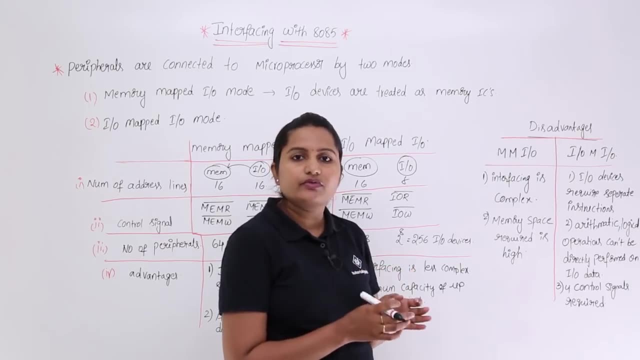 so coming to memory mapped io mode, the disadvantages are: interfacing is complex because we need to get clarification. so coming to memory mapped io mode, the disadvantages are: interfacing is complex about which is io which is acting as memory and what is the actual memory. so that's why interfacing 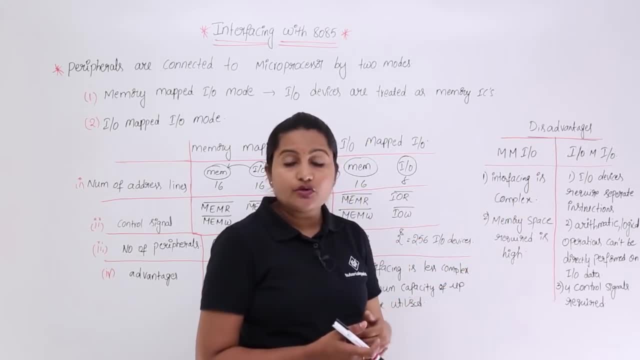 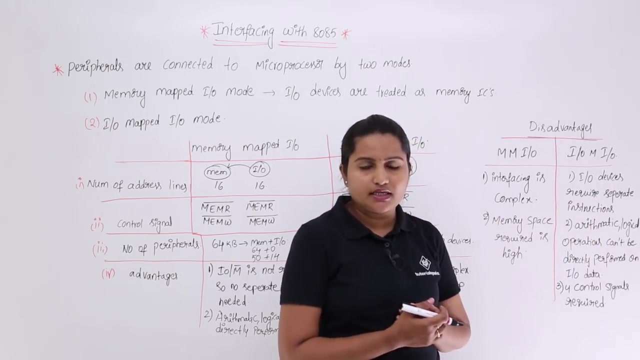 is complex and memory space required is high, so we require high memory space. as we are using io is also as memory, so we require memory as high. so here, coming to io mapped io, io devices require separate instructions here, why? because we are not using io as memory, we are using io separately, so separate.